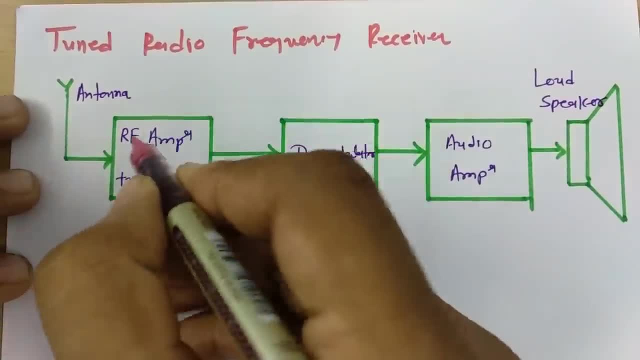 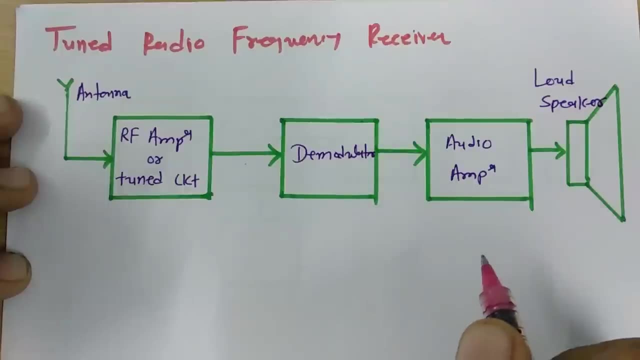 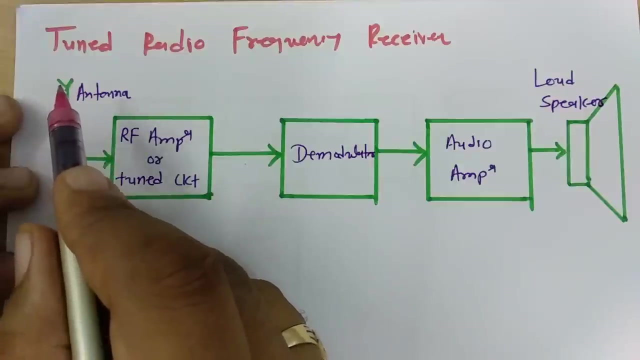 Welcome to analog communication playlist. Here in this session I'll be explaining tuned radio frequency receiver And this is basic block diagram of it, where first element is antenna that will be receiving almost all frequency components and that will be given to RF amplifier or tuned circuit. 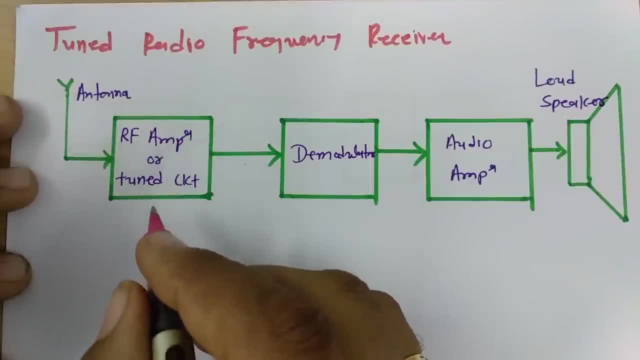 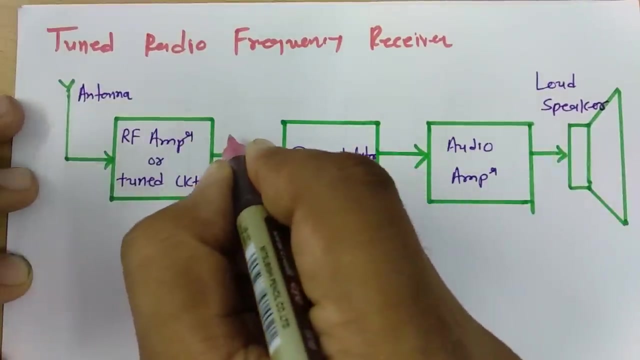 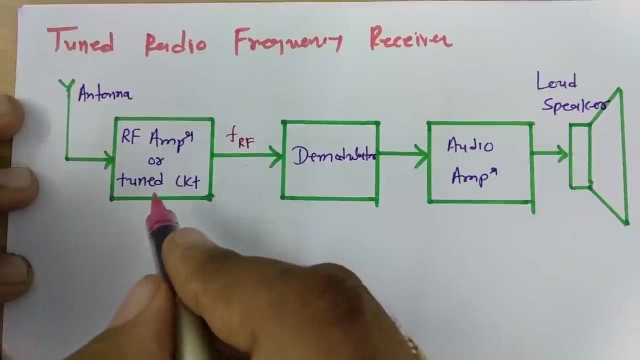 This RF amplifier, or tuned circuit that is made up of inductor and capacitor, and this circuit that will be receiving RF signal and it will give it to demodulator. So over here you'll be finding RF frequency components are there and that frequency components are tuned by tuned circuit and this tuned circuit that is basically made up of: 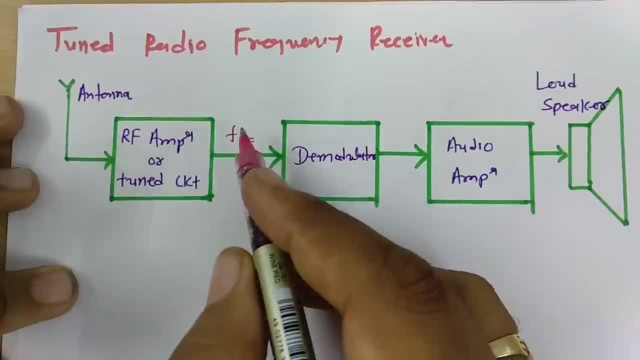 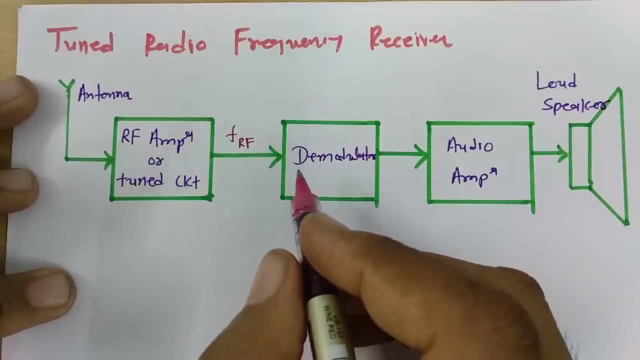 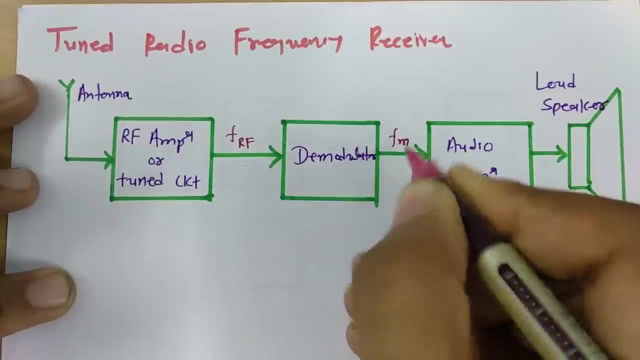 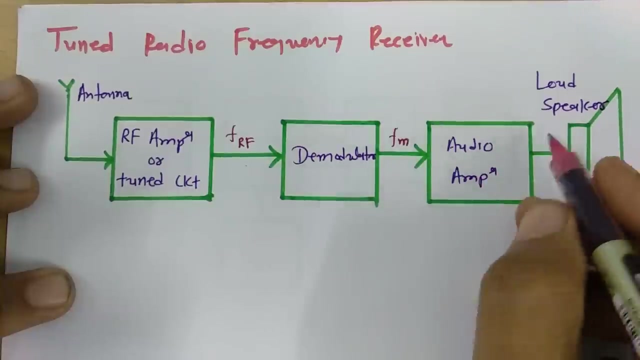 Inductor and capacitors And then after this RF signal that will be given to demodulator circuit, In demodulator circuit it will be extracting message signal. So over here there will be message signal that will be weak message signal and after amplification of that message signal we will be giving this message signal to loudspeaker. 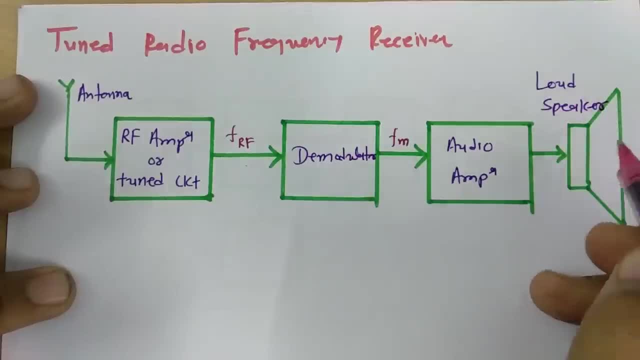 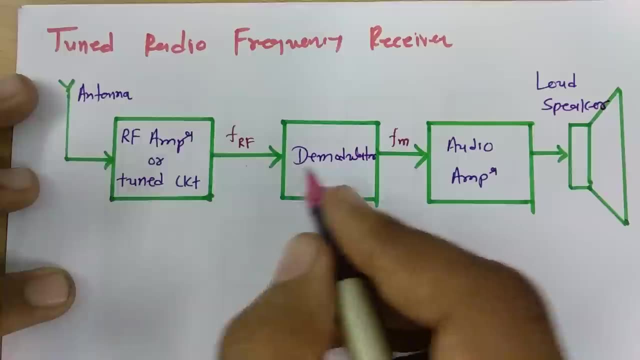 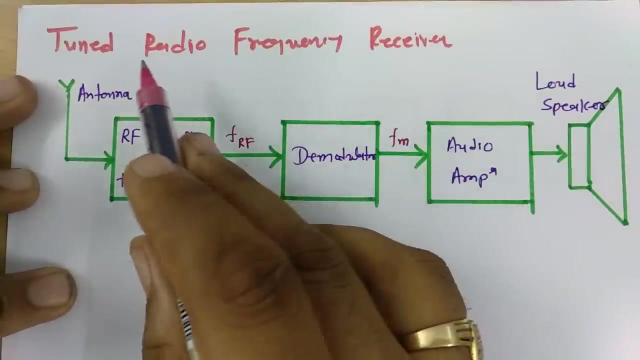 So that we can have that Voice in speaker with larger amplitude. Now basically there could be question like: what is there which is there inside of this demodulator circuit? So for that, if I give you one basic example like: see, here we have this tuned radio frequency receiver as AM receiver. 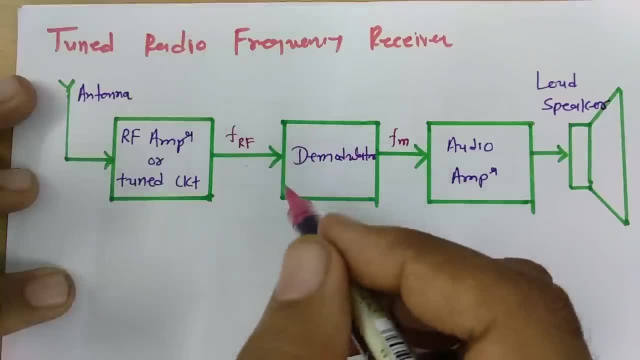 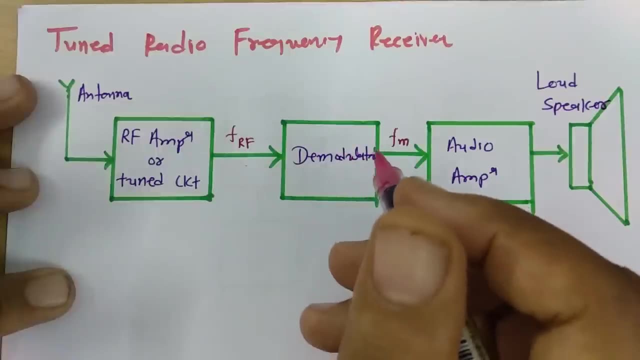 So in AM receiver here there could be envelope detector, And in DSBSC as well as SSB- I have already explained so many demodulators. And in DSBSC as well as SSB. I have already explained so many demodulators. 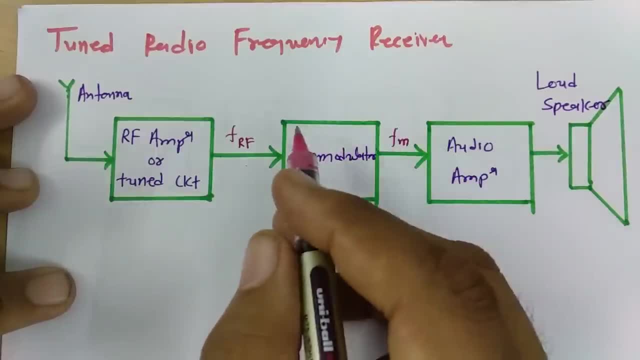 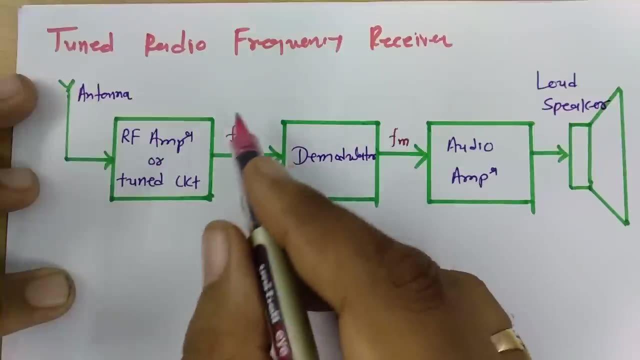 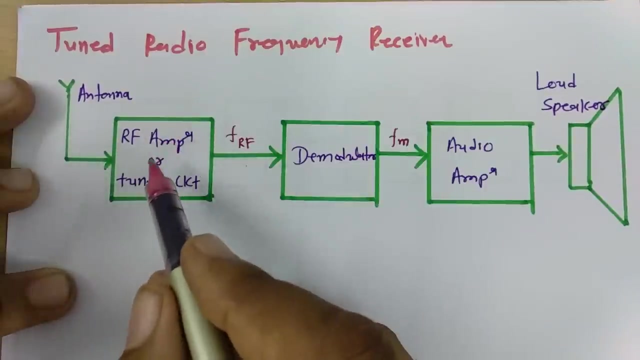 So out of all those demodulator there could be any demodulator which will be extracting original signal from modulated signal. So here this antenna will receive so many frequencies, here tuned circuit that will be tuning particular frequency with particular bandwidth. 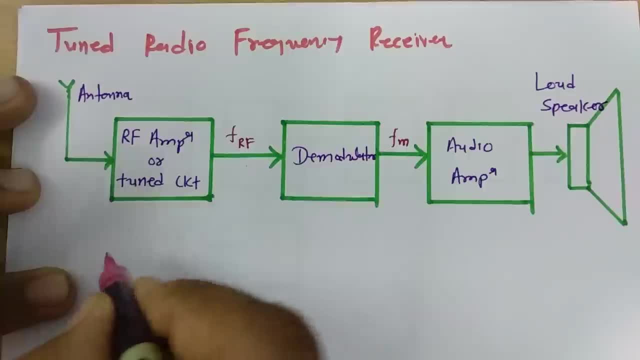 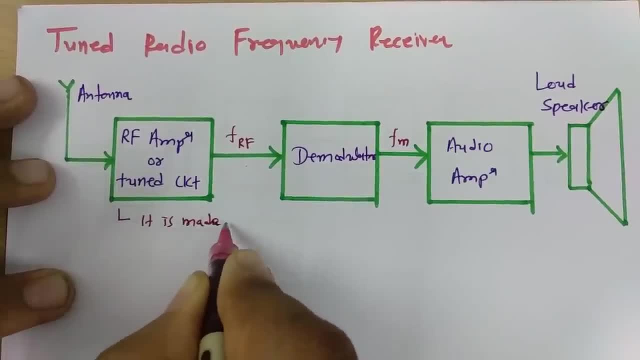 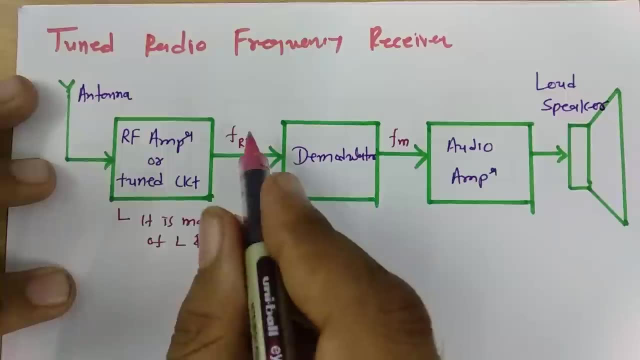 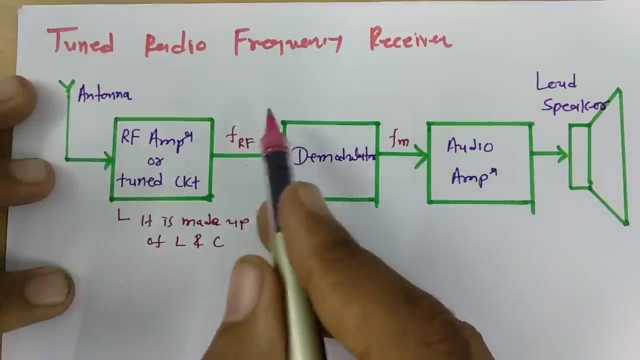 it is made up of inductor and capacitor and that will tune particular frequency, that is RF frequency. now, once you tune that to particular frequency, will be having demodulator circuit which will extract msg signal out of modulated signal and then, after we just give it to amplifier circuit. 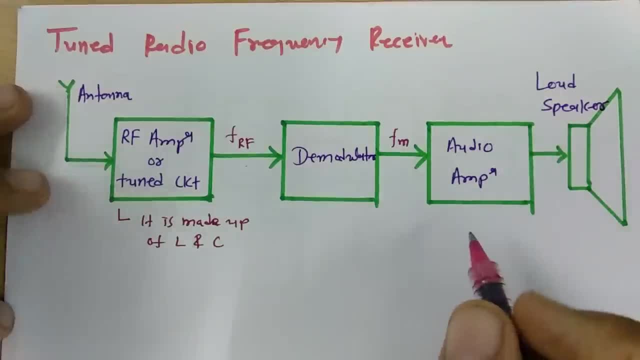 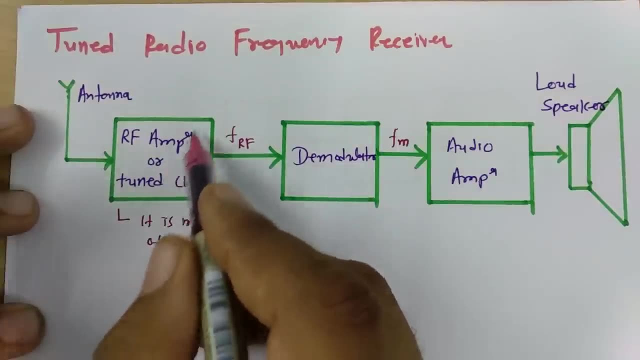 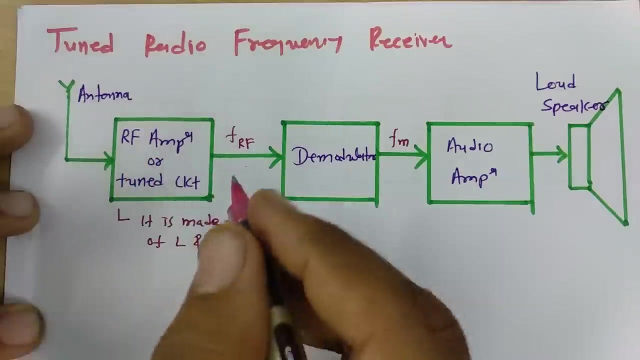 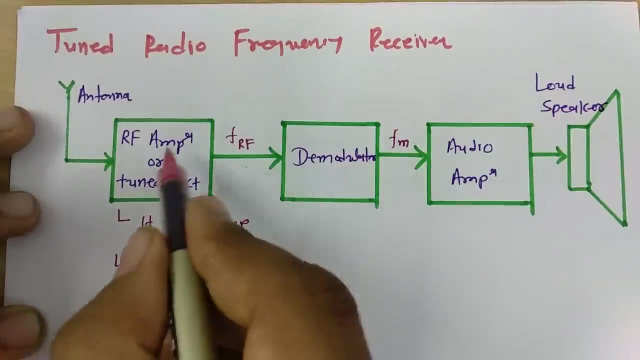 and then after we just give it to amplifier circuit and then it will be given to loudspeaker. now here, basically, this circuit, tuned circuit, this will be justifying quality of received signal and that quality of received signal that is based on quality factor. so quality factor, quality factor of this received signal that is based on center, 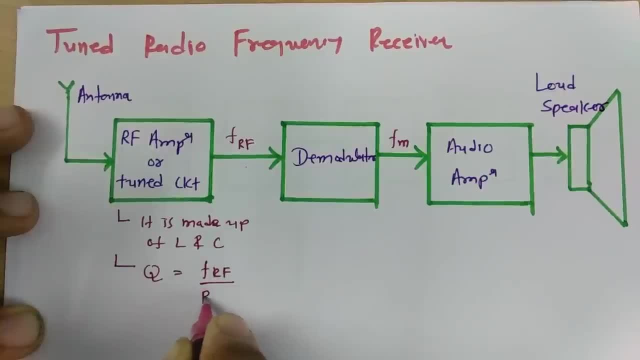 frequency of rf divided by bandwidth, and here for am broadcast, for am broadcast this range of rf frequency that is there in between 550 kilohertz to 1650 kilohertz. so these many parameters that is there with this demodulators that we have already. 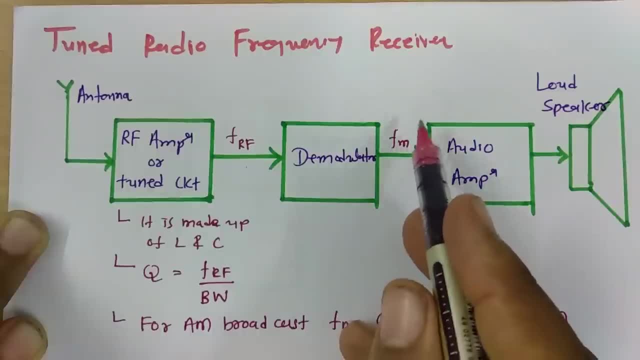 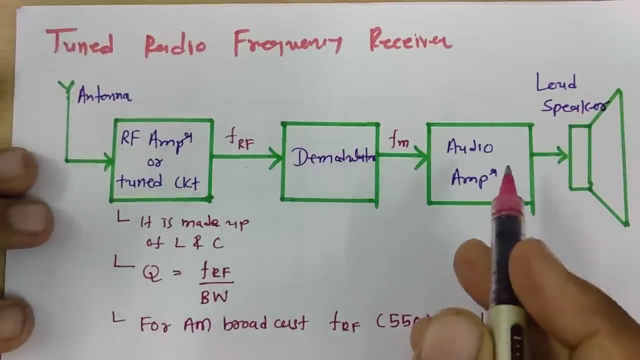 studied for am. then, after you will be having weak message signal, you just give it to audio amplifier and then that could be given to loudspeaker. now there are a few issues that i would like to discuss here. so to understand those issues, let us have one example. so 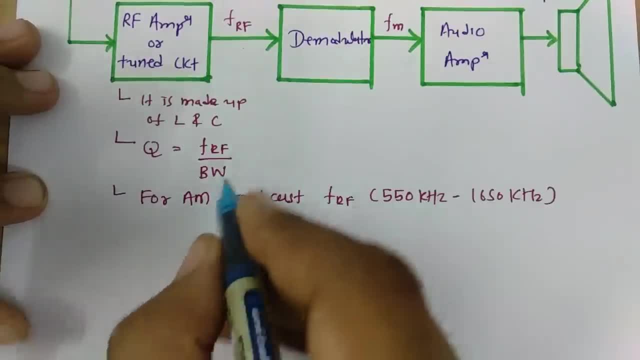 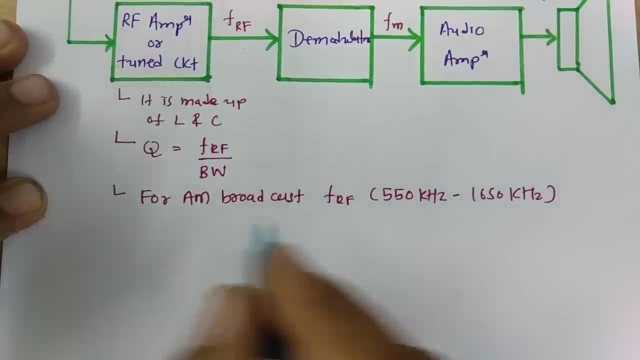 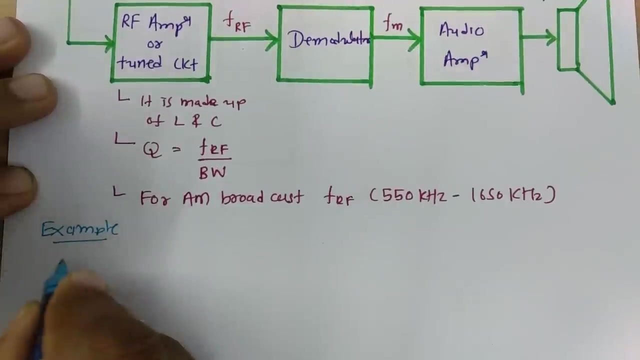 here, as i have told you this, for this am broadcast frequency range. that is there from 550 kilohertz to 1650 kilohertz. so i'm just considering one case where, if i say i have rf signal out, of this am that is tuned at 1000 kilohertz. 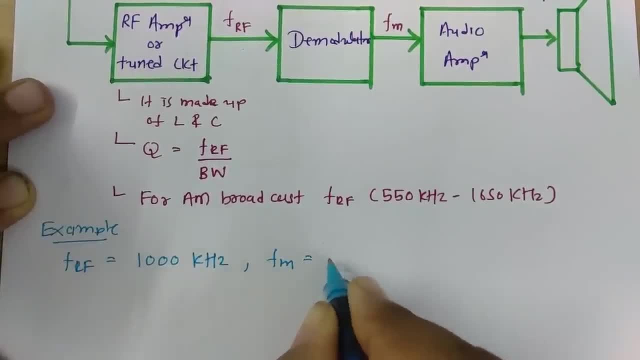 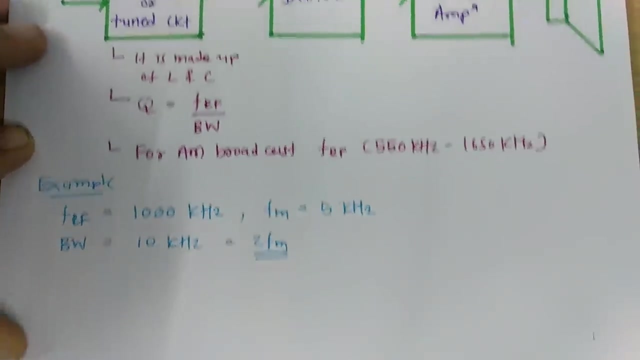 and my message signal that is having frequency of 5 kHz and if I say my bandwidth, that will be 10 kHz. for AM, as we know, it is 2 FM, so as per that it will be 10 kHz. So, based on that, if we 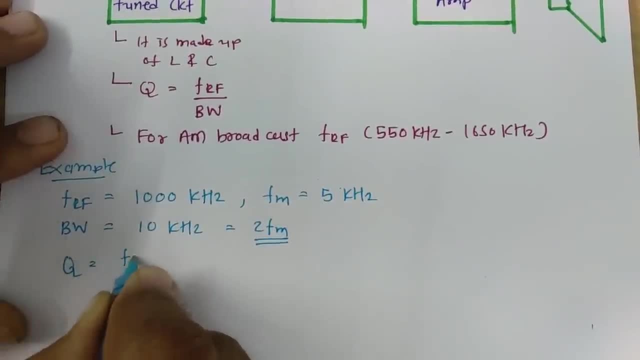 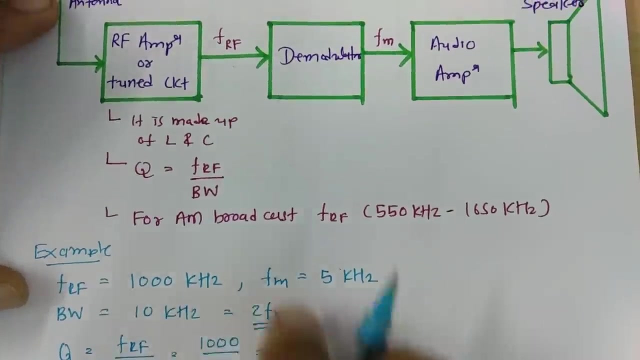 calculate quality factor, then quality factor is center frequency, that is 1000, and bandwidth, that is 10 kHz. So this will be 1000 divided by 10 kHz, that is 100. So quality factor is 100 over here. Now, when we talk about this 100 quality factor, it is extremely difficult to design such 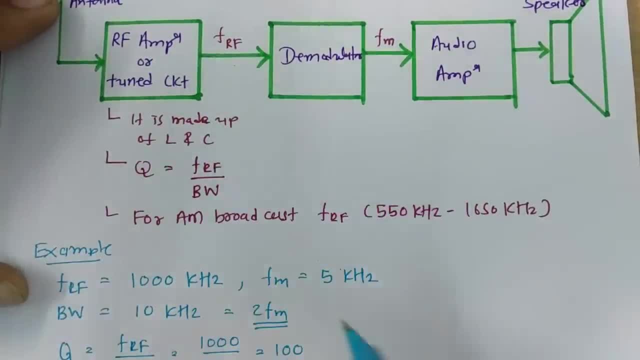 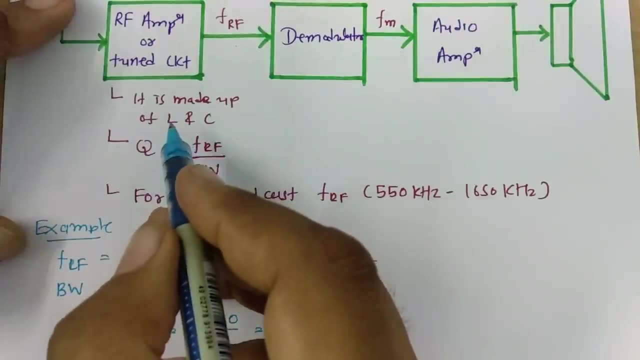 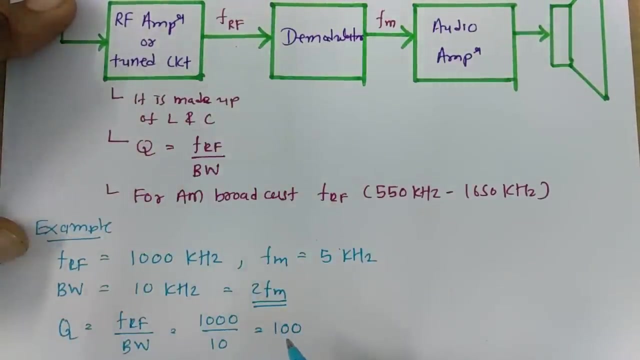 tuned circuit and RF amplifier To have quality factor of 100. So when we talk about this components- inductor and capacitor- it is extremely difficult to design those tuned circuit which is having quality factor which is somewhere around 100.. Now I just want to explain few problems which is happening. 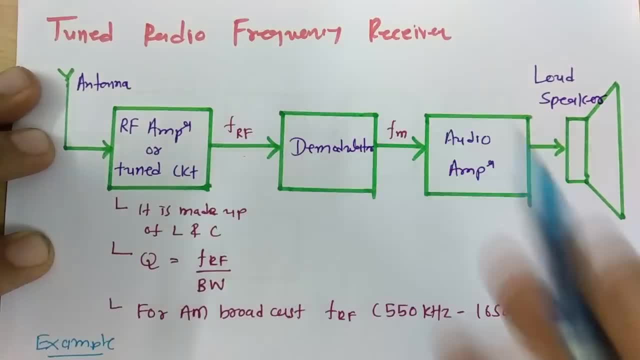 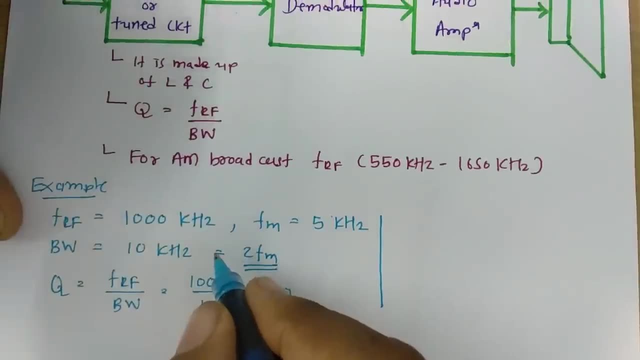 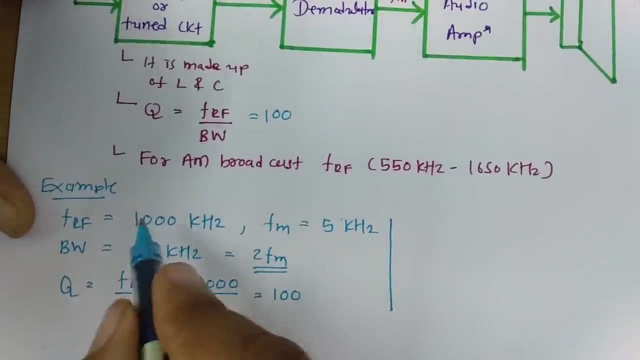 by this tuned radio frequency receiver. So, to understand those problems, let us have fix quality factor. Now, if I say I have quality factor with this circuit, that is 100.. And that is to receive the signal that I have already explained. Now, if I consider 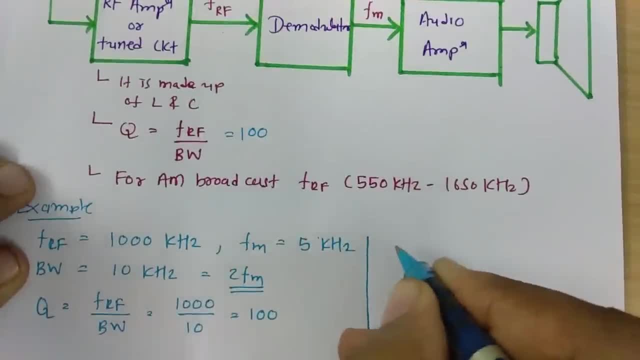 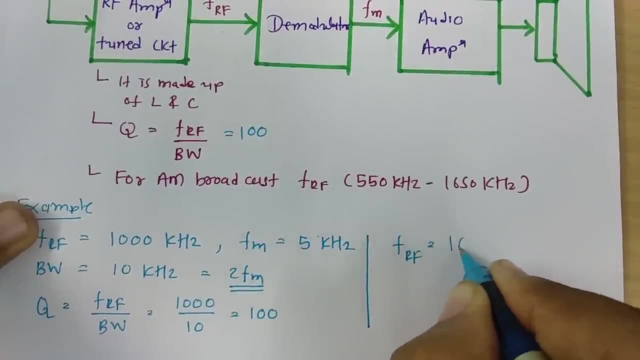 my quality factor is 100. and now if I retune this to other frequency, that is RF frequency, that is 1600 kHz And already I have told quality factor is 100. so in that case if you see bandwidth, so that bandwidth that will. 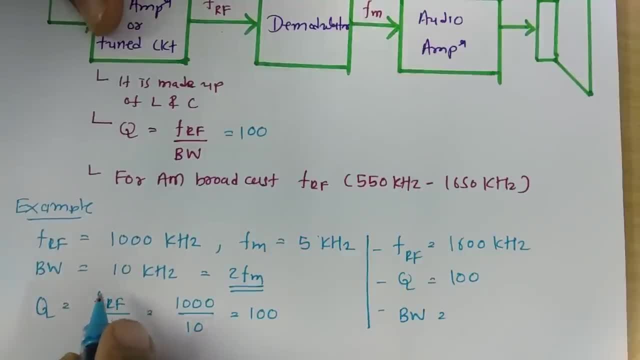 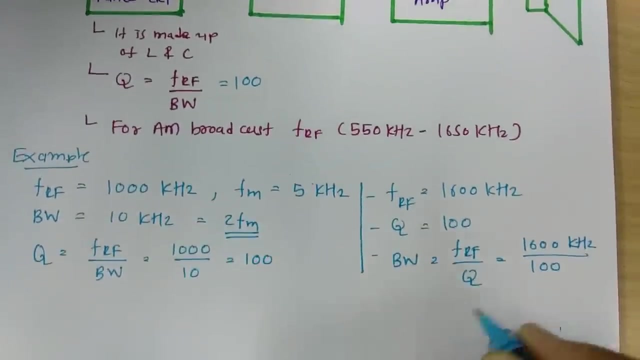 be, as per this basic formula, bandwidth will be radio frequency divided by quality factor and radio frequency over here that is 1600 kilohertz, and quality factor that is 100. so here we will be having bandwidth of signal that will be 16 kilohertz. so here one can. 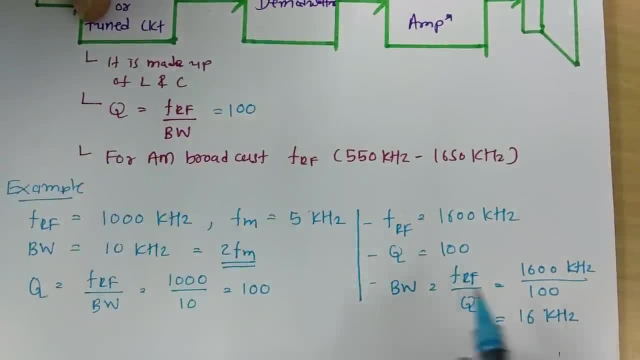 see, as if you tune this circuit to higher frequency, received bandwidth will be higher. in this case it is 16 kilohertz initially. we have defined for message signal by 10 kilohertz, so even we design circuit with quality factor that is 100 sometimes you will be receiving 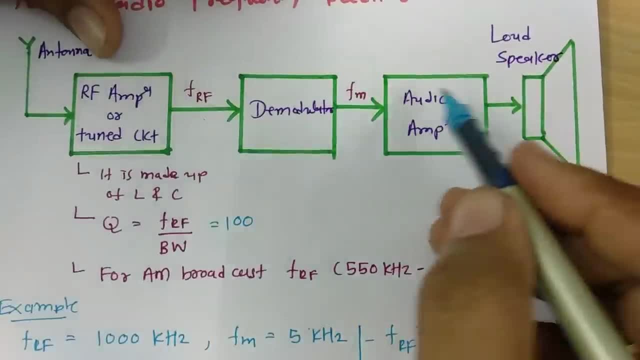 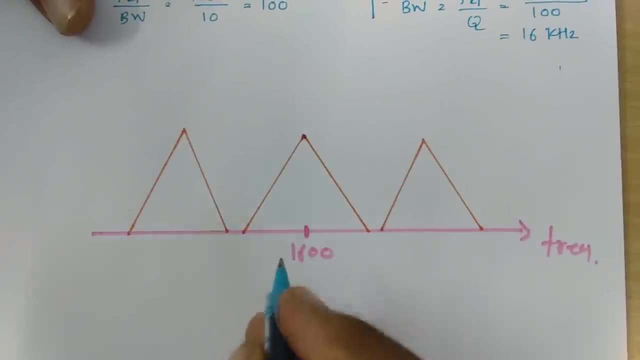 signal with bandwidth of 16 kilohertz. over here you will be receiving signal with bandwidth of 16 kilohertz, so let us try to understand that. on frequency plot, so when I say this is what my 1600 center frequency and if it is having bandwidth received by 16 kilohertz, 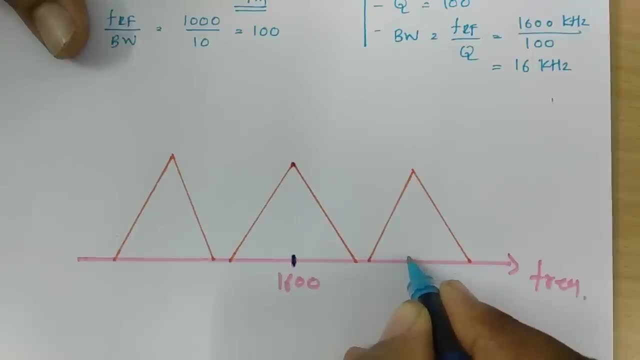 then 16 plus 8 kilohertz over this side and 1600 plus 8 kilohertz over this side and 1600 plus 8 kilohertz over this side signal will get received. so over here it will be 1608 kilohertz and over here it will be. 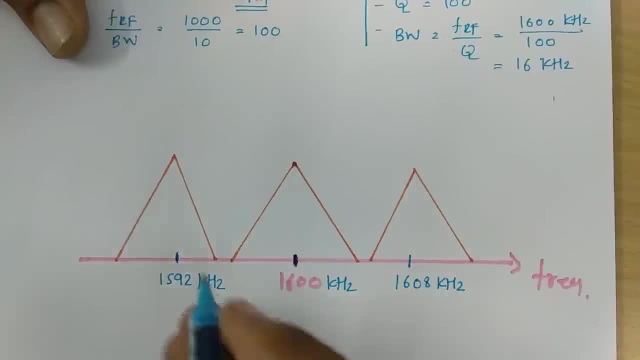 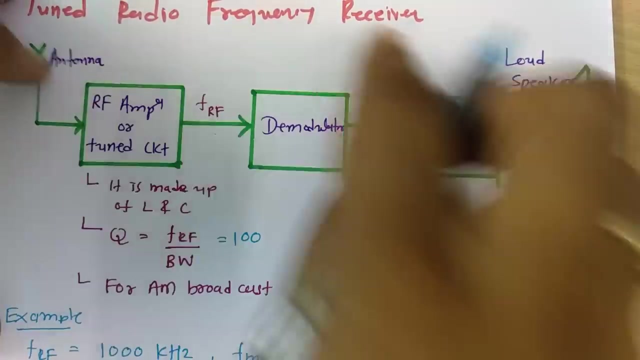 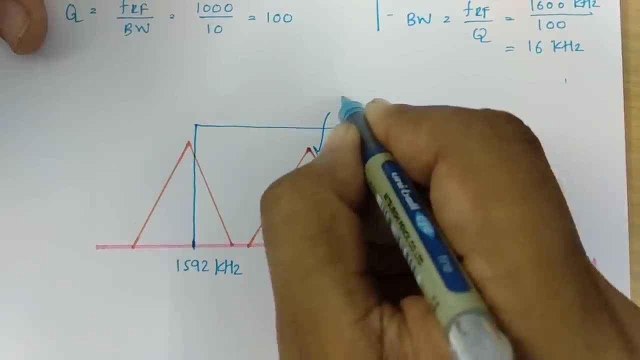 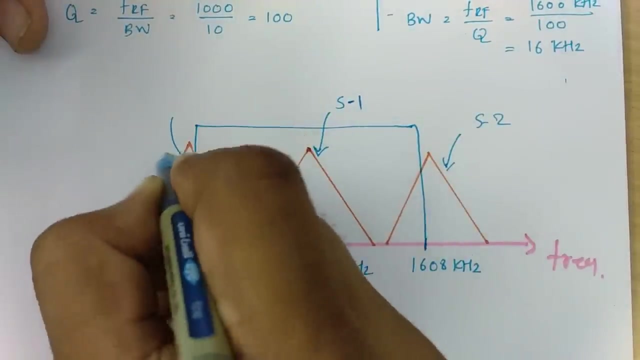 1592 kilohertz. so probably you will be observing, this will be a signal which we are receiving. this will be a signal which we are receiving by this tuned radio frequency receiver. now, here one can see, this is what my station one, let us say, this is station one, this is station two and this is station three. now, because 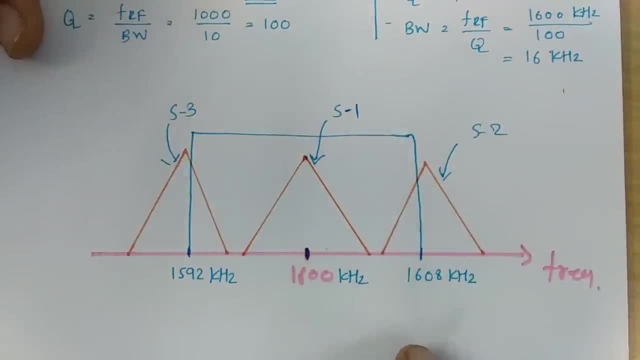 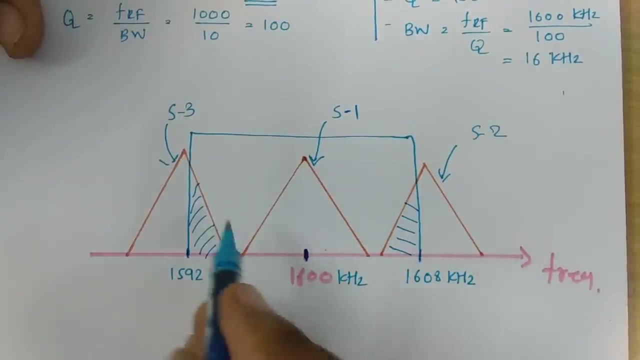 of bandwidth received, which is 16 kilohertz. you will be finding, even though you tune this circuit to center frequency receiver by this tuned radio frequency receiver now here one can see that is 1600 kilohertz other stations portion that will get included at receiver side. so you will be finding this. 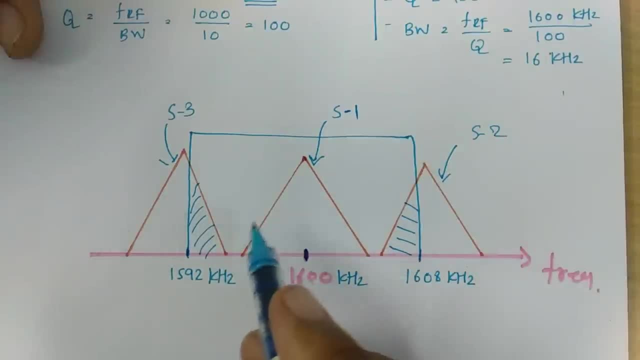 is what adjacent station signal which is what we are receiving, even though we tuned this circuit to this station. so this is adjacent channel interference. so here one can see adjacent channel interference is happening by this tuned radio frequency receiver. now, here one can see adjacent channel interference. is happening by this tuned radio frequency receiver. now here one can see adjacent channel interference. so this, an adjacent channel interference, this is what my station will receive when its been tuned尼 by this tuned radio frequency receiver. now here one can see adjacent channel interference is ending. 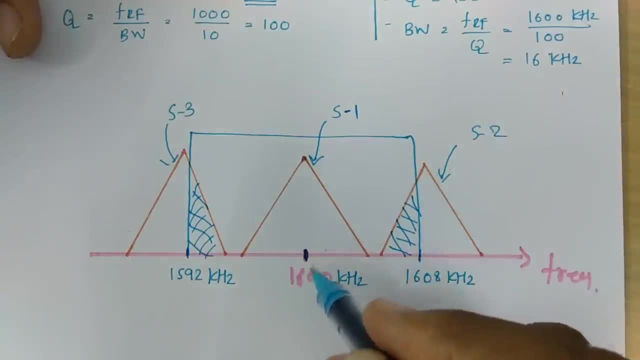 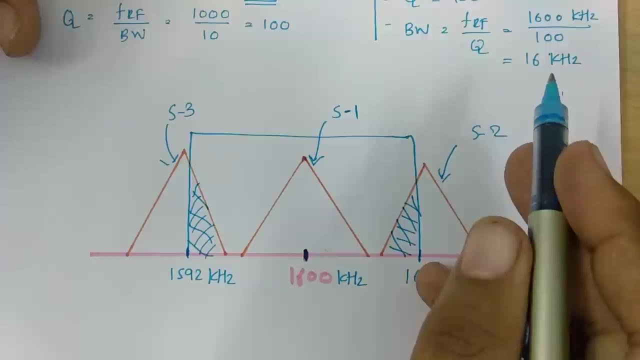 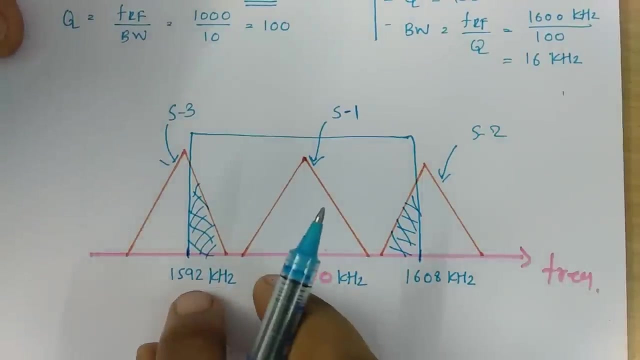 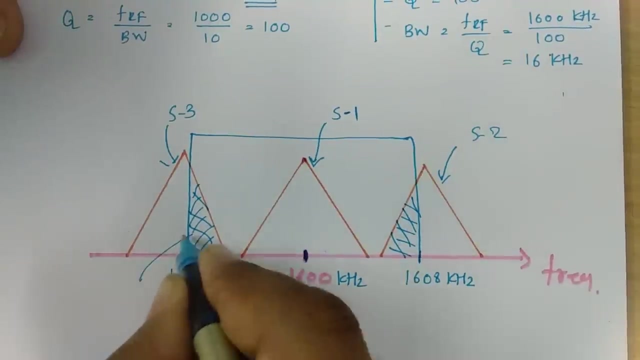 settings assessed. okay, now, only so. you are showing a segment. so if you are making a told, that is the noise. so how do we operate? what are you going to do when we make a known based and running circuit, then why you should do inci here. I just want to explain here, maybe giving you an example of what you can do with. 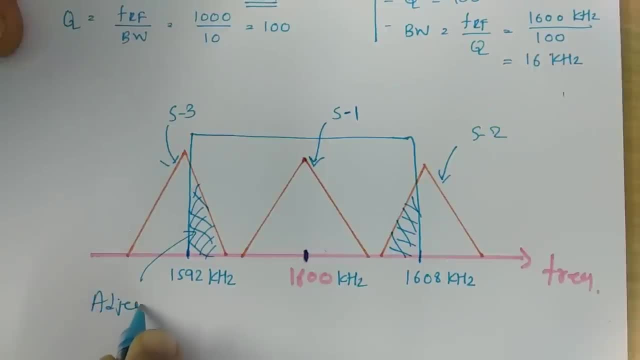 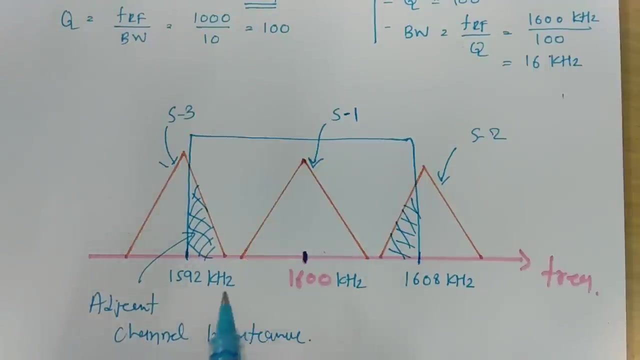 this is this: if you go to this bottom line of the cute one color, you have a radio frequency and because of this problem we don't use this radio receiver so often. but this problem could be resolved by super hydrogen receiver, so that i'll be explaining in next session, so just stay. 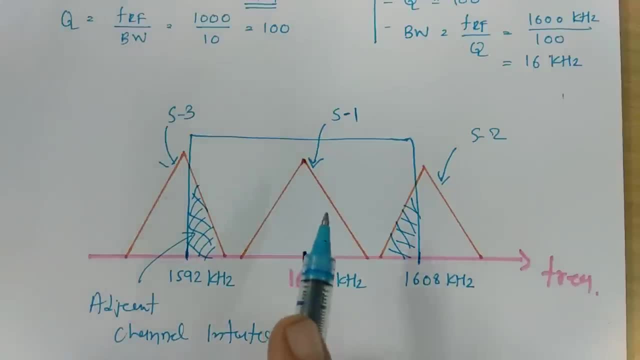 tuned with this channel. i'll explain how we can resolve this problem. so here one can see, selectivity is not good. as well as you'll be finding, there will be adjacent channel interference because of improper selectivity and quality factor is not good enough over here. so to have scalable quality factor we can go for super hydrogen receiver. so that is what i'll be. 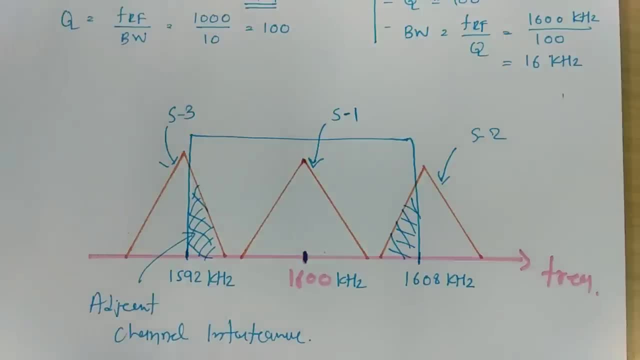 explaining in next session. just stay tuned with this channel and you can give me your valuable suggestions. thank you so much for watching this video.